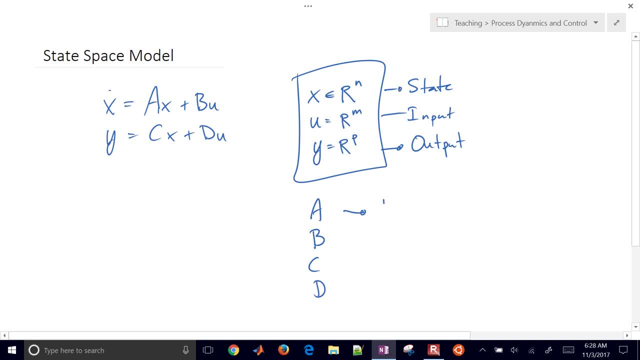 And this one, the A matrix, is going to be an N by N matrix. The B matrix, This is going to be an N by M And the C is going to be a P by N And the D matrix will be a P by M matrix. 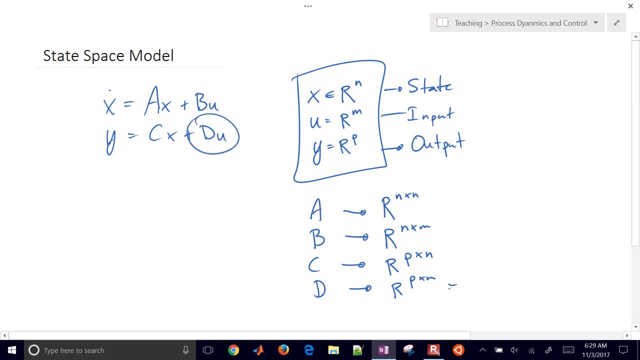 Now the D matrix is typically just equal to zeros, And often the C matrix is just one of the states, Or sometimes it's just the Identity matrix. Okay, if you have all of the states being measured, So most of the information that we 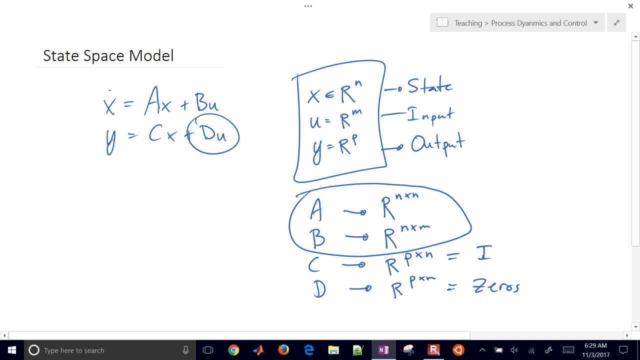 When we derive these is typically in the A and B matrix, And these are just the output equations. So let's talk about some of the things that we can derive from these. So first of all, we can look at stability And we can just take the eigenvalues. 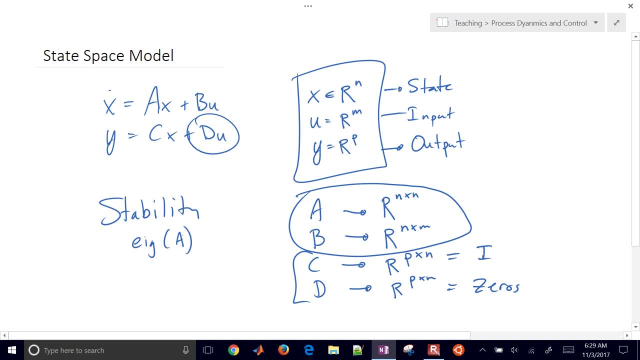 Of the A matrix And see if the system is going to be stable or not. And it's going to be stable if all of the eigenvalues have real components that are negative. So we have the real components of the eigenvalues. If they're less than zero, then we're going to be stable. 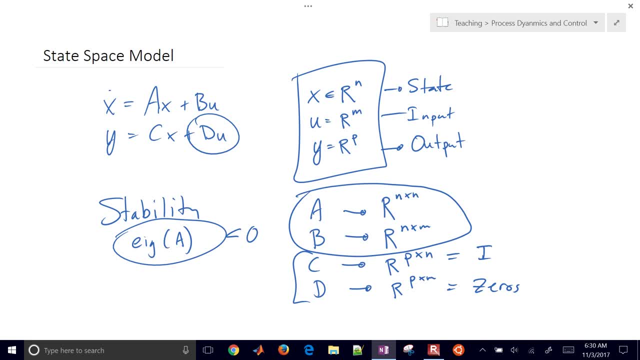 But if any of them are greater than zero Or equal. If it's equal to zero, then it's an integrating system, And if it's greater than zero, then it'll be unstable. Okay, so let's just do an example. 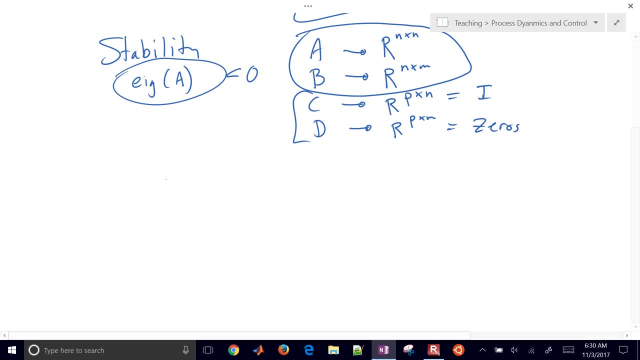 Now let's do a simple example with just a first order system. So let's say we have a differential equation that looks like this- This is a common description of many dynamic systems With a gain and a time constant. So this is our gain. 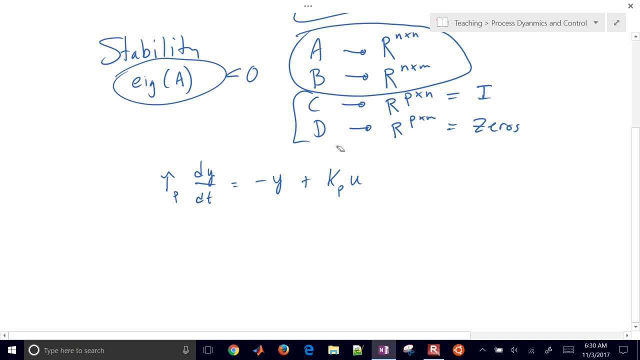 And that's our time, constant, And just putting this into state space form. We would just rearrange this And create a state x, So we'd have x, dot, Or that's dx, dt Equals, And then I'll go ahead and divide through. 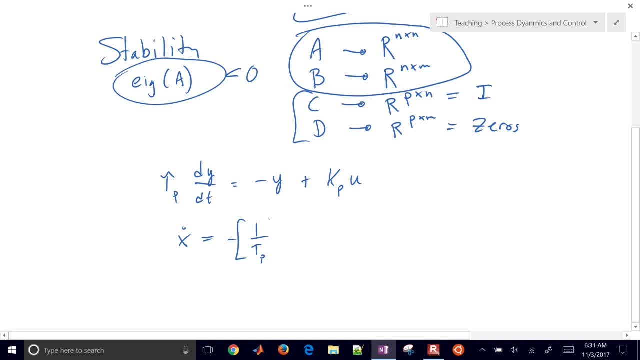 The tau p value Times x Plus kp over tau p Times u, And then just create my output, Which is y equals x. So this original equation right here in state space form Becomes two equations, And then my a matrix is just going to be a one by one. 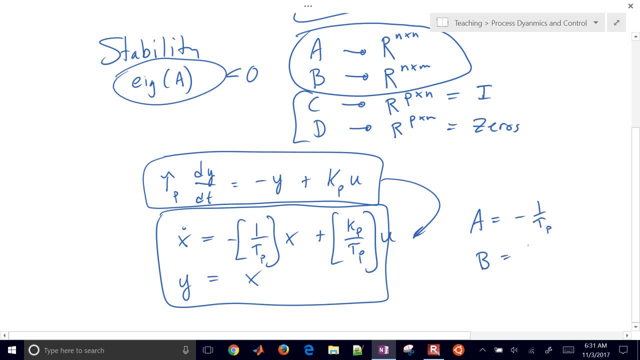 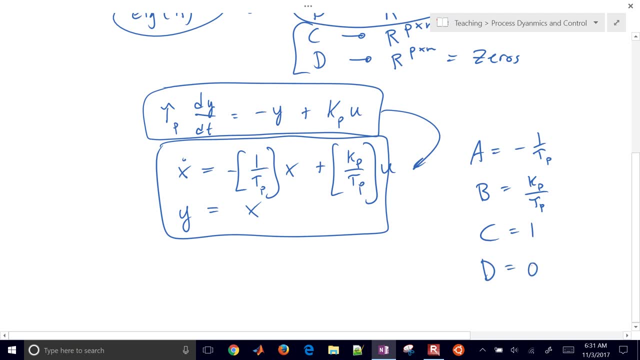 And it's going to be minus one over tau p. My b matrix is going to be kp over tau p. C equals one And d equals zero. Okay, so here is my state space Representation of that system. Let's do this for a second order system as well. 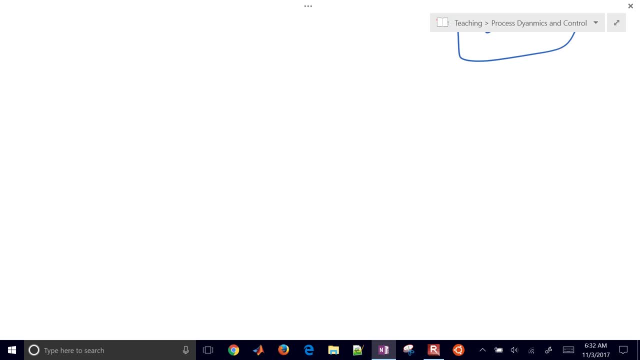 So let's say we had this original equation that we just discussed, Tau p, But now I'm going to have a second one as well. So I'll do tau p one Equals minus x, one plus kp times u, And then I'll have a second one. 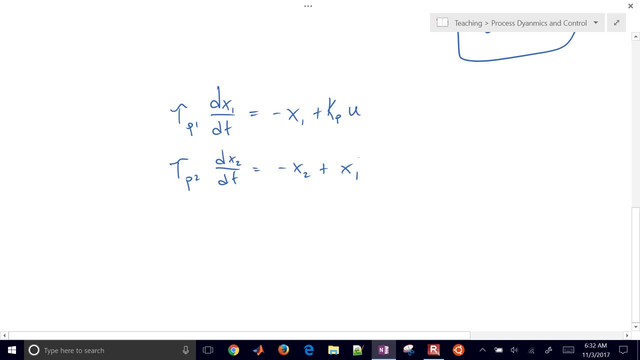 Okay, so just two equations. This is a second order system, And then we'll have our output as well. This is just going to be our second state. So if I divide through by tau p one and tau p two And then just rearrange this, 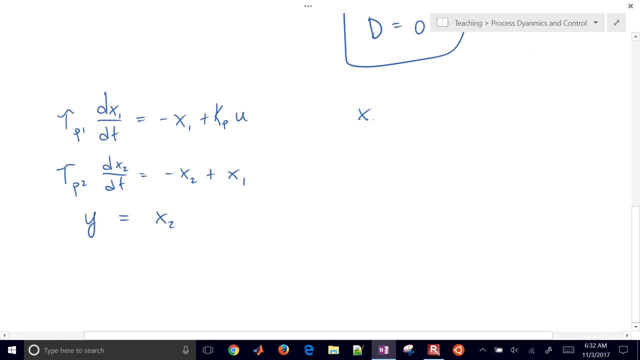 I'm going to put This into the state space form, Where I'd have x one dot and x two dot. Those are the derivatives with respect to time. And then here is my a matrix, And that's going to be minus one over tau p one. 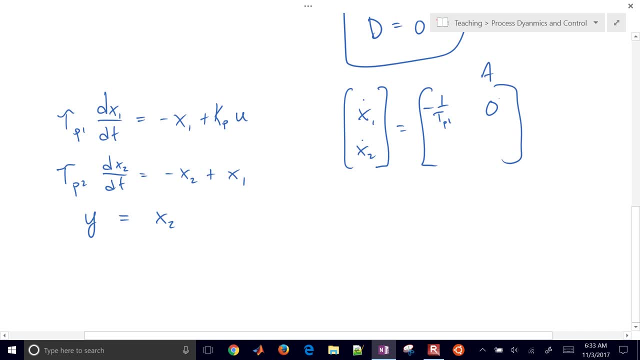 And then I'll have a zero here, Because I don't have x two in my first equation, And I'll write this in matrix form. And then I'll also have one over tau p Two and minus one over tau p one or tau p two there. 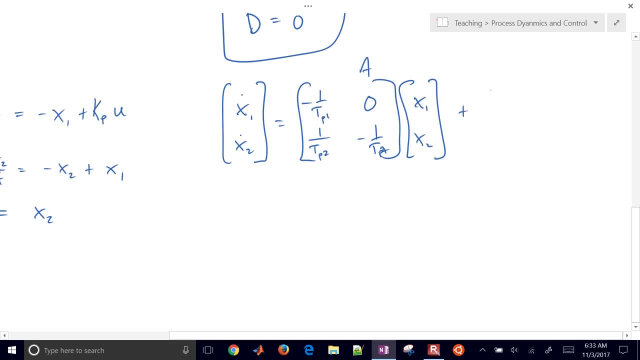 Okay, so we have: there's our a matrix And then our b matrix is going to be kp over tau, p one, And then zero there, Because we don't have u in our second equation. And let me go ahead and just there's my y equals. 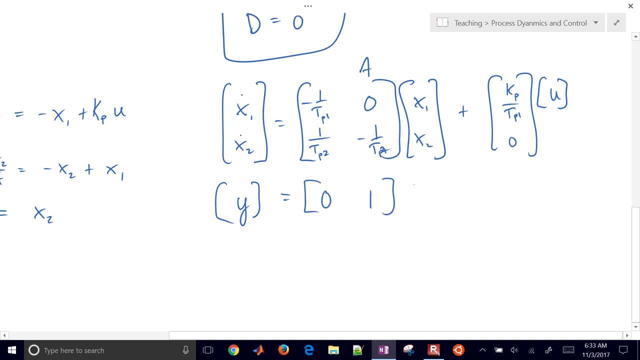 And then I have my c. So that's going to be the matrix, And that's multiplied by x one and x two, So this one's just: y equals x two Plus zero times u. Okay, so here's a, b, c and d matrices. 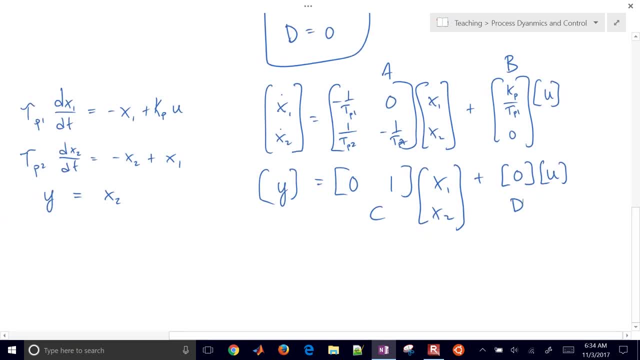 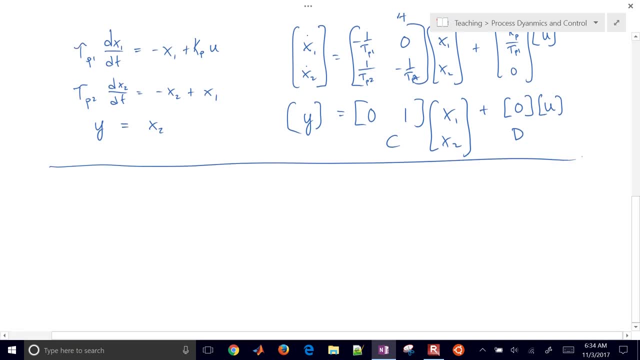 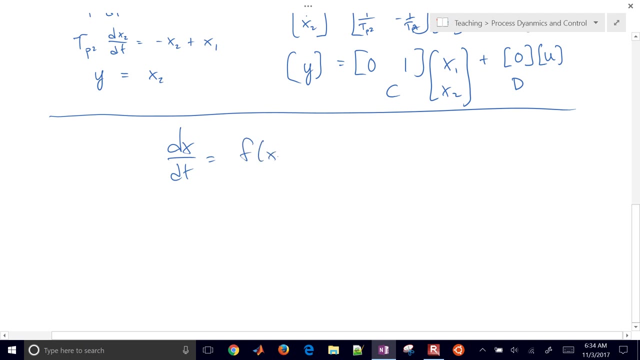 So I've put this one into this State space form. Okay, let's talk about just general non-linear systems. So let's say you have dx, dt equals f of x and u, and then y equals g of x, and we want to translate this into state-space form. 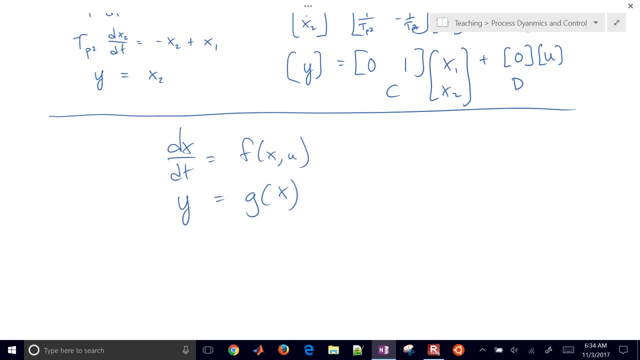 So if this is general nonlinear, then we need to linearize it. So we're going to linearize the right-hand side of this and that's going to be approximately equal to: And if we choose steady-state conditions, then our nominal values will give us zero derivative. 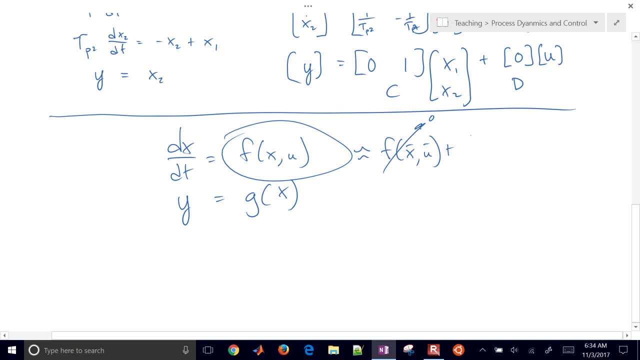 That will be equal to zero. And then you need to take the derivative with respect to x, plug in the nominal values and then you can do x minus x-bar. x-bar is the nominal value, And then you'll also have df du. 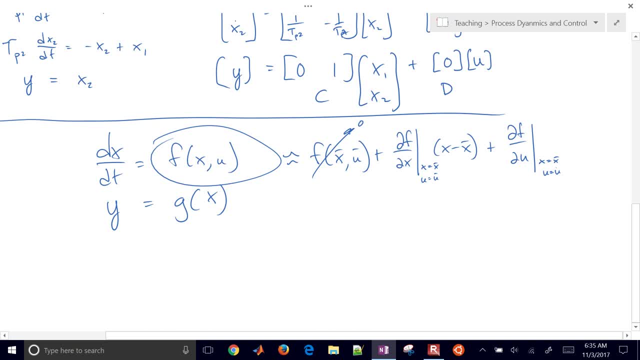 Plug in the nominal values again, And then this will be u minus u-bar. So this right here will just be a number, and I'll call that alpha, And this will just be a number, I'll call that beta. And then we also want to linearize this one. 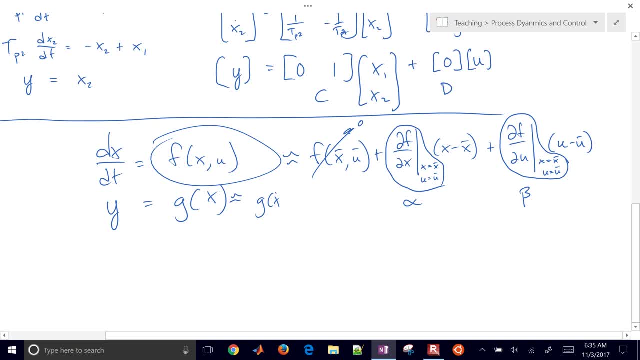 Okay, so that's going to be g of plug in the nominal values plus, and then we'll take the derivative of g with respect to x and plug in the nominal value there. Okay, and I'll call this one right here. I could call that gamma, for example. 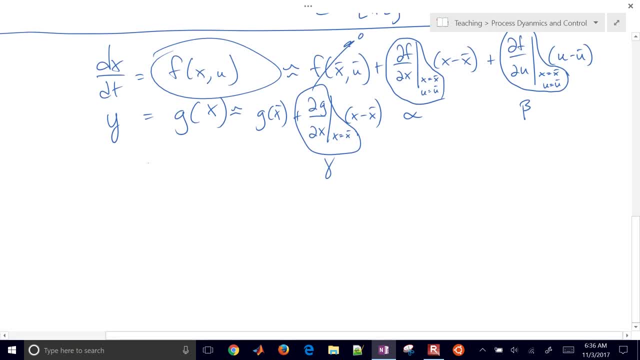 Okay, so in state-space form, then it would come up with something like this, where we would have alpha times x- I'll call that x-prime for deviation variable. Okay, I'm in deviation variable form plus beta times u-prime. 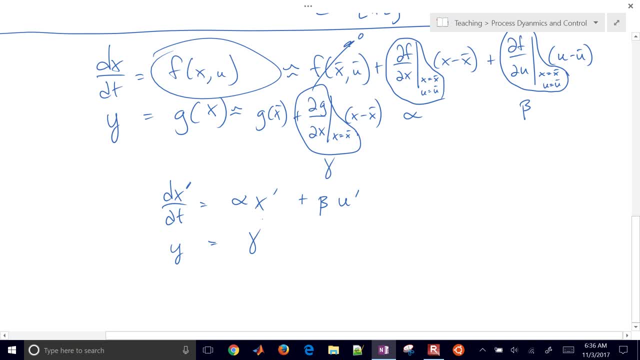 And then I'll have: y equals gamma times x-prime. So this would be my A matrix, this would be my B matrix and that would be my C matrix. So I've translated any general non-linear system into state-space form. 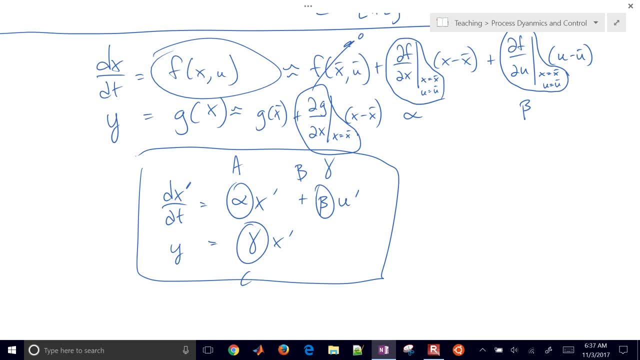 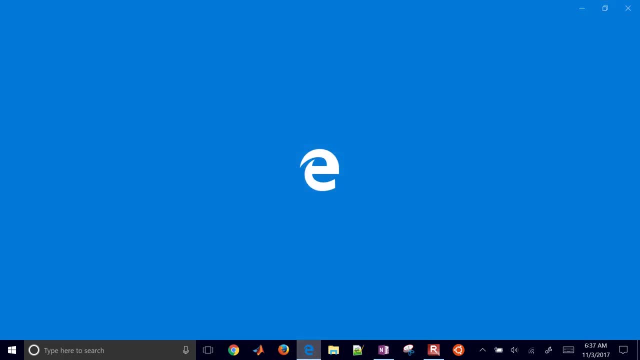 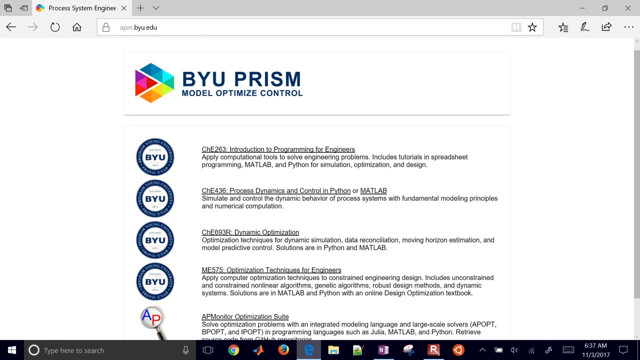 And if you have additional states there, you can just take the partial derivative with respect to those states or those additional inputs. Okay, So just some additional content on this. if you just come to apmonitorcom, this is listed under the process dynamics and control course. 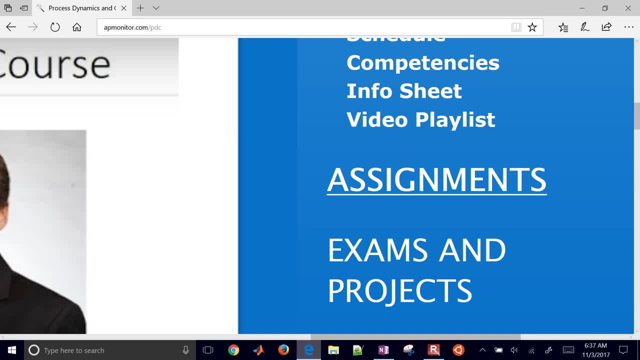 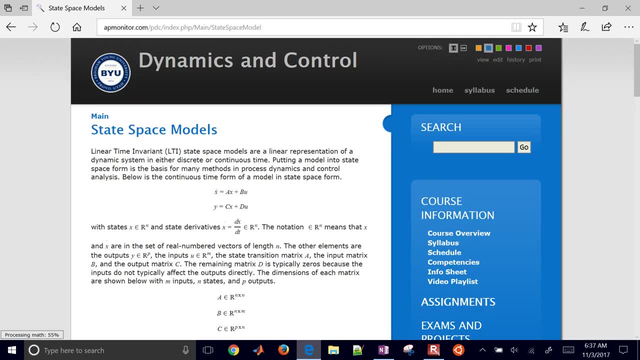 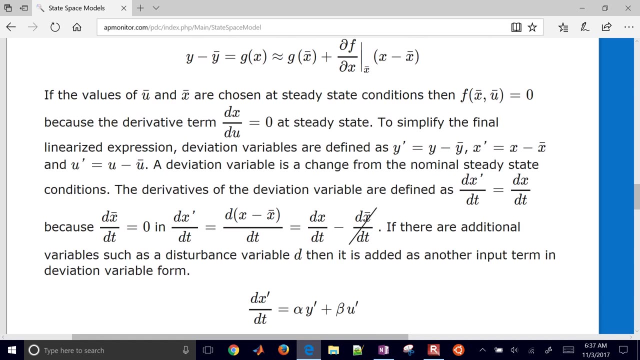 And if you go down to assignments, you'll see an assignment on this as well, but also some additional material on state-space models, the information that we just showed here on state-space models, And then a number of examples as well. Okay, so here's the general non-linear system for state-space. 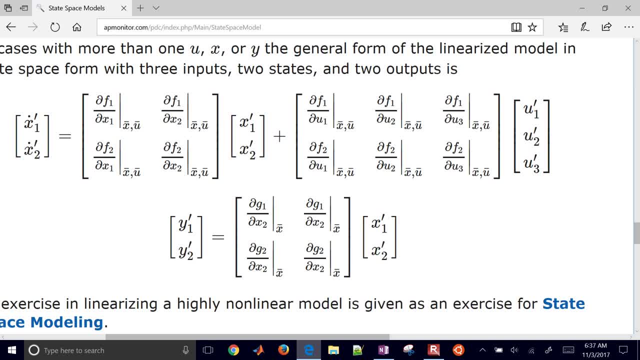 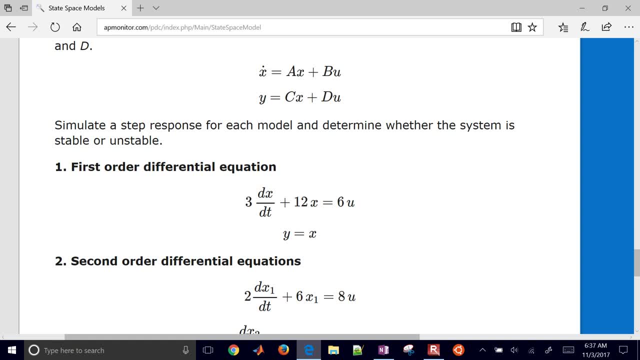 As I mentioned, you just take the derivative with respect to each variable and then put it into this matrix form. And then here are a few exercises as well. You have one through four here. Here's the first one, just putting this one into state-space form. 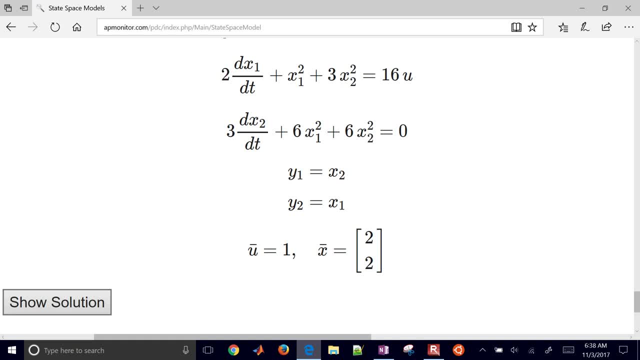 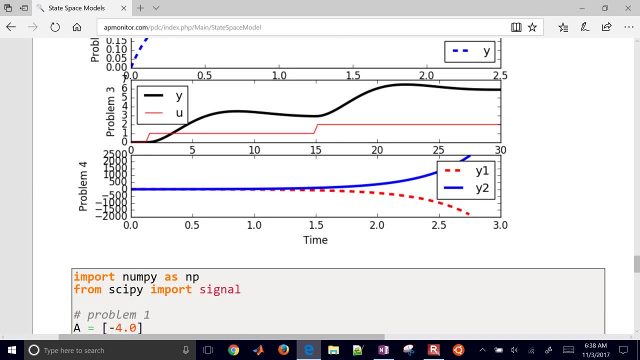 And then it gradually gets a little bit more complicated. Okay, Here's the final one. If you'd like to see the solutions, just select this. There's another video there and it'll show you the solutions with some source code in Python. 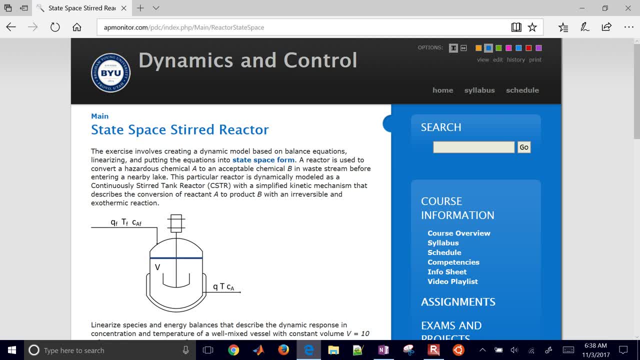 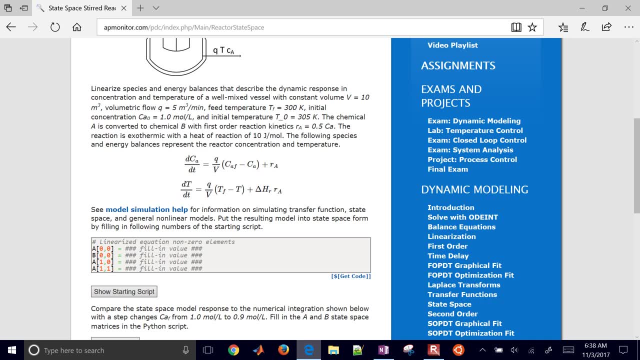 And then, finally, you have the. this is going to be the next exercise that we'll do. This is a state-space stirred reactor, And you need to derive the state-space model and then simulate it.